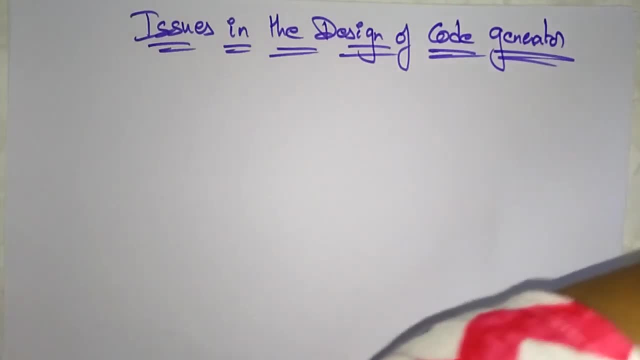 students, welcome back now. coming to the next topic, that is, the issues in the design of the code generator. so so far we had seen different phases in the compiler design, so we reached the end of the subject. you know you already learned the concept of lexical analysis, syntax analysis. 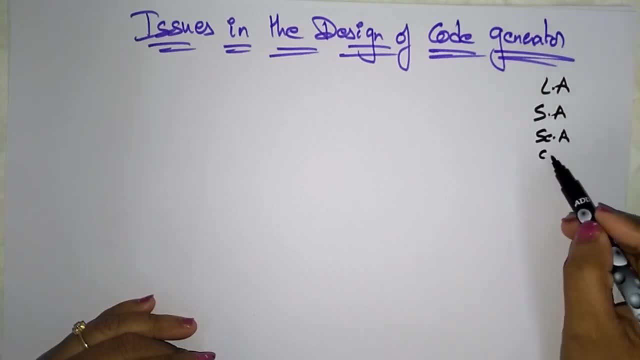 semantic analysis, okay, the code intermediate, code generation and the code optimization. now let's see the code generator. that's a code generator. if you want to design a code generator, you need to follow the some rules and the other issues that were you are facing while you are. 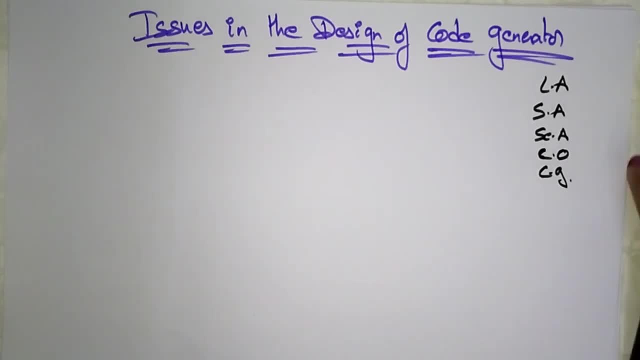 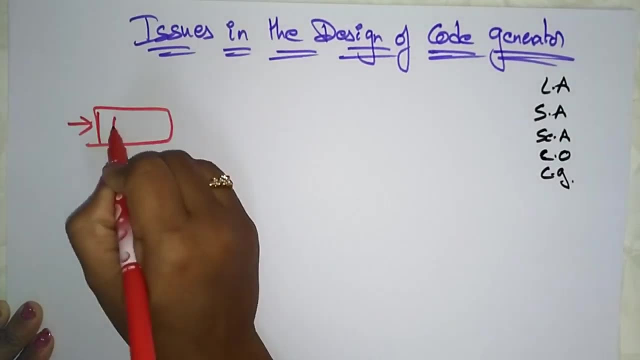 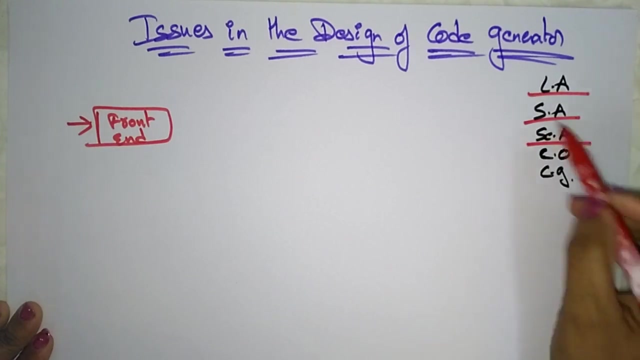 designing the code generator, where the exactly the code generator will be seen. so let's see the position of the code generator. let's take the front end. so the front end is nothing but the less: lexical analysis, syntax analysis and semantic analysis. so this comes under the front end. so the front end giving the source. 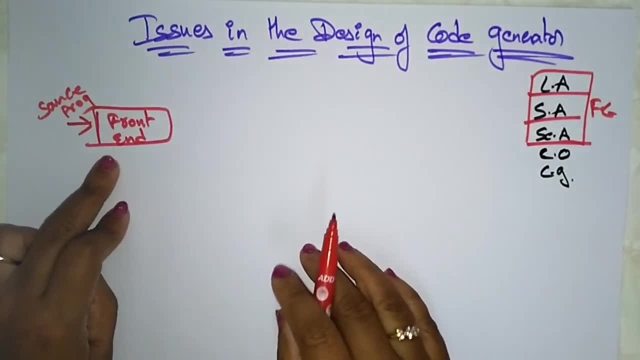 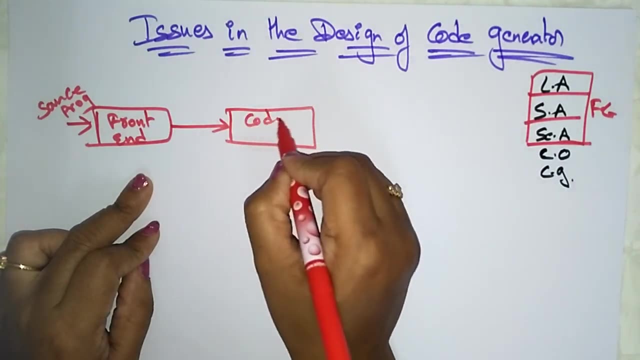 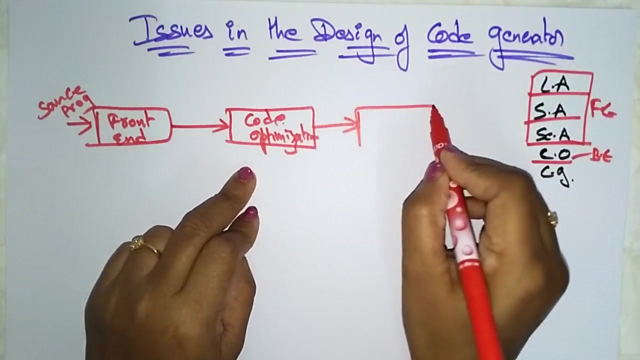 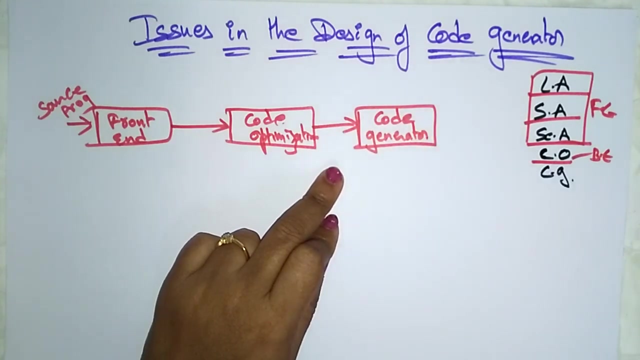 program input is the source program. okay, so the front hand to code optimization. so the code optimization, the code optimization is the back end, the code optimization. okay, so the code optimization to code generator. so here the position will be there, the code generator and the final you'll get. 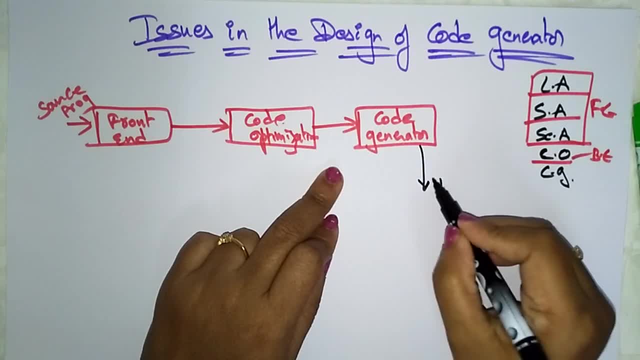 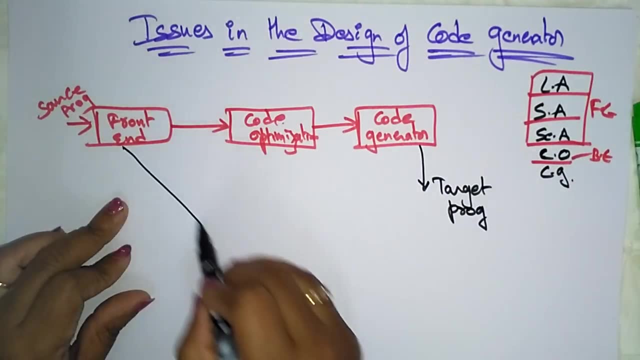 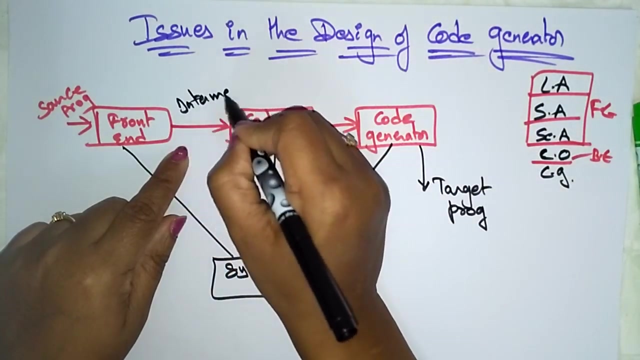 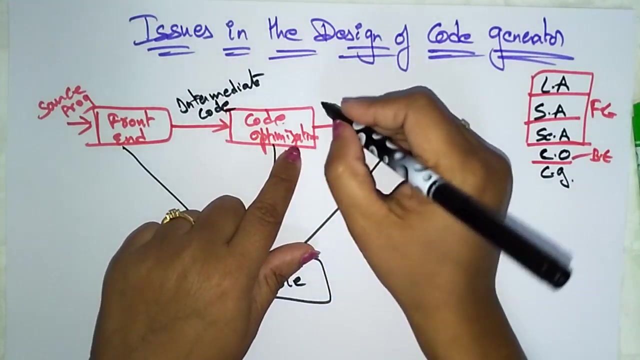 from code generator, you'll get the target program. you reach the target program, which is assembly level language. okay, so here everything will be connected to the symbol table. symbol table: okay, so the front and is generating the intermediate code- intermediate code, which is ready for the execution, and the code optimization is also generating the intermediate code, intermediate code. 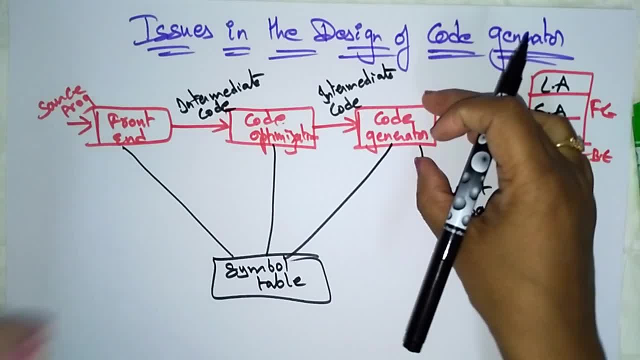 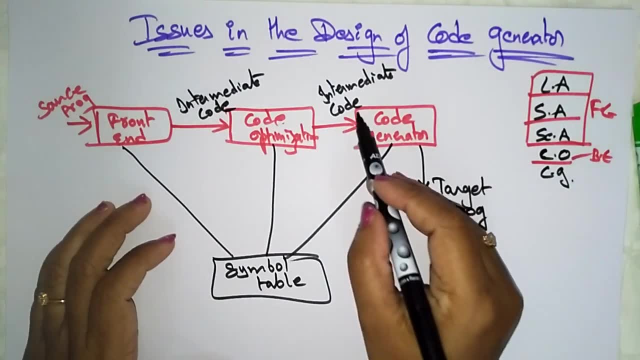 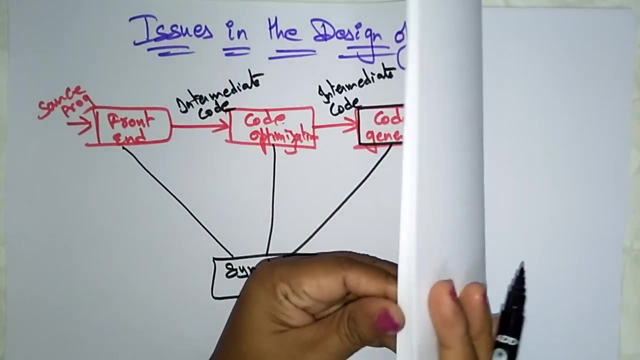 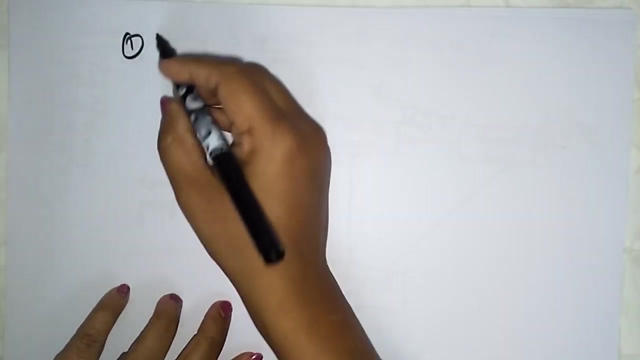 to code generator and the code generator will take the intermediate code and finally gives the target program. so this is the exact position of this code generator. Now let's see what are the design issues in this code generator. The different the designs issues in the code generator is: first thing, input to code generator. 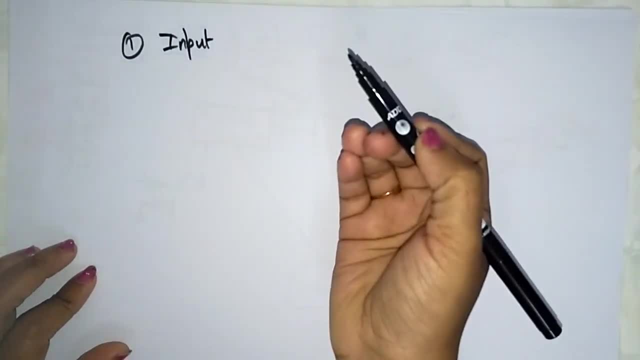 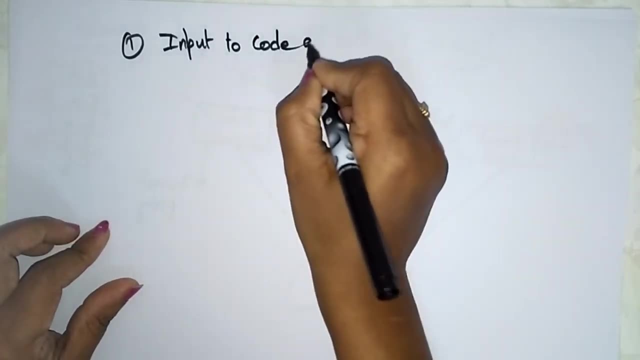 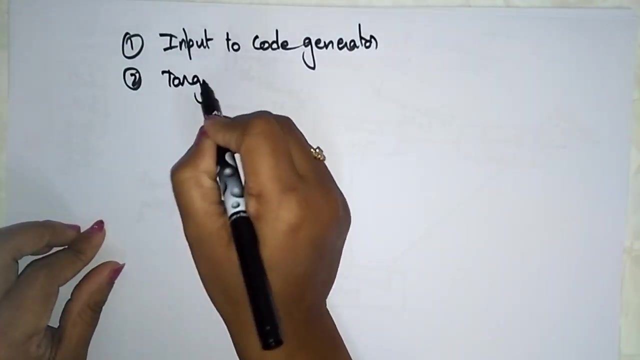 First design is: first, you have to give input to the code generator. that is nothing but the intermediate code. you are giving input to the code generator. Input to code generator. and the second: you have to know the target program. you have to reach the target program. 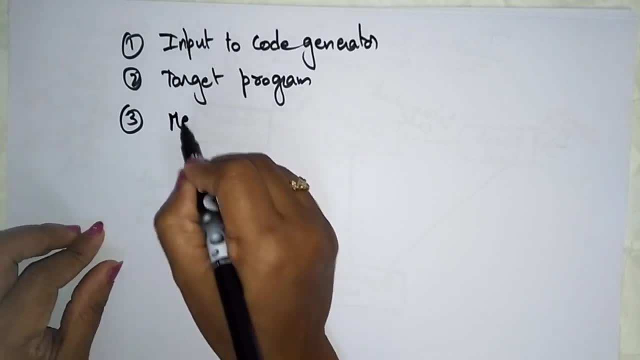 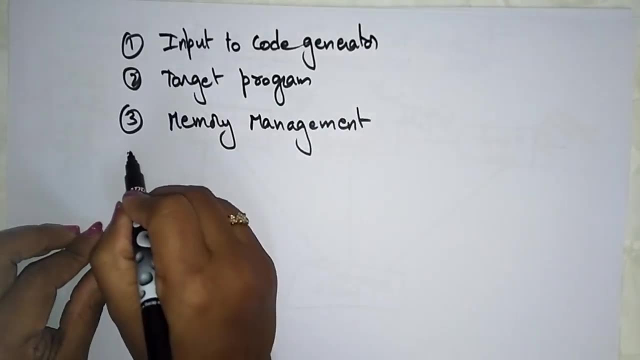 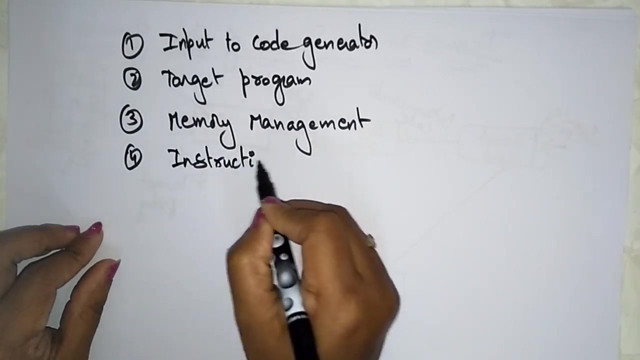 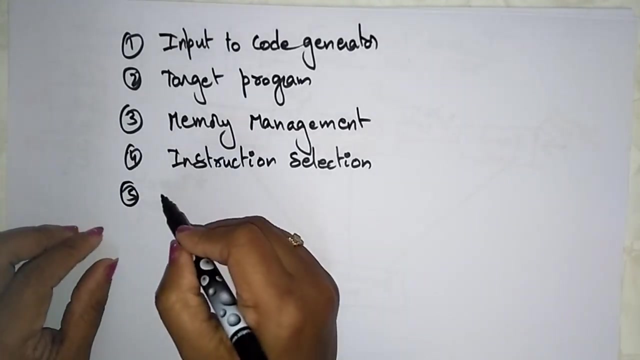 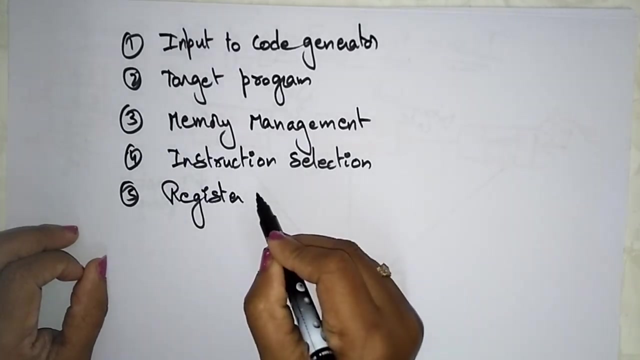 Third design issue: memory management. how the memory is going to be managed in the code generator memory management. Fourth one: instruction selection. what type of instruction it has to be selected to support the code generator? Fifth one: register allocation issues. is there any register allocation issues? are there register? 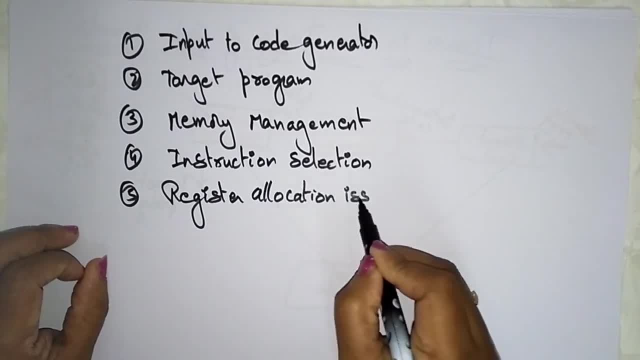 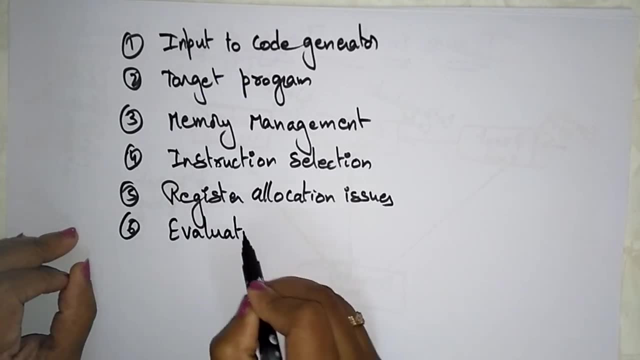 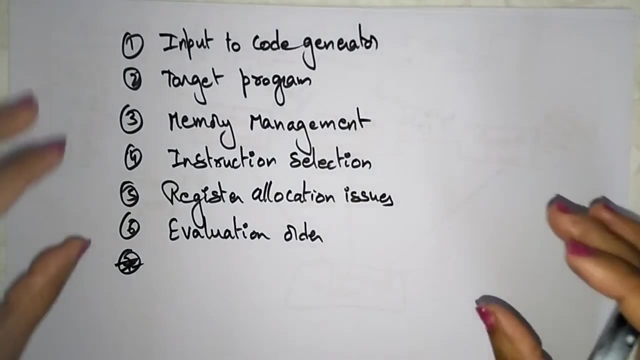 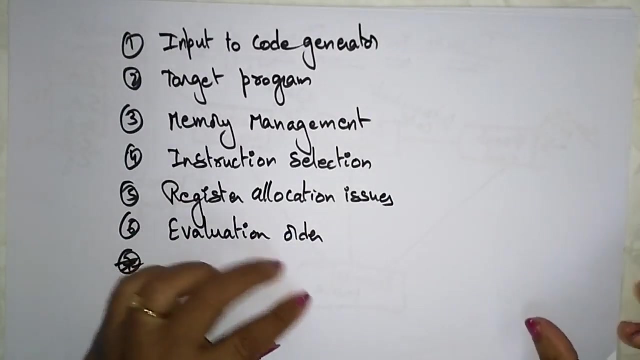 allocation issues. evaluation order. evaluation order. so which order you have to follow to evaluate The expressions, and okay? so these are the six design issues. issues in the design of the code generator, let's discuss one by one. so the first design issue is the input to code generator. 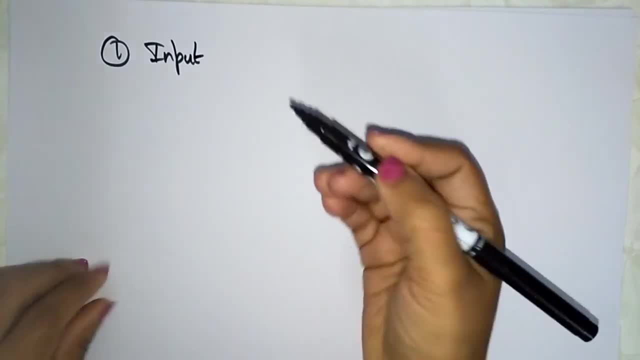 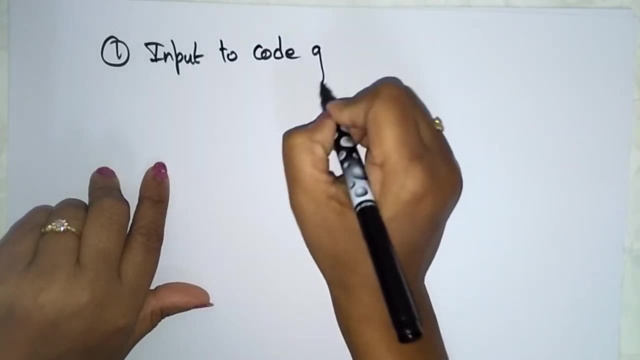 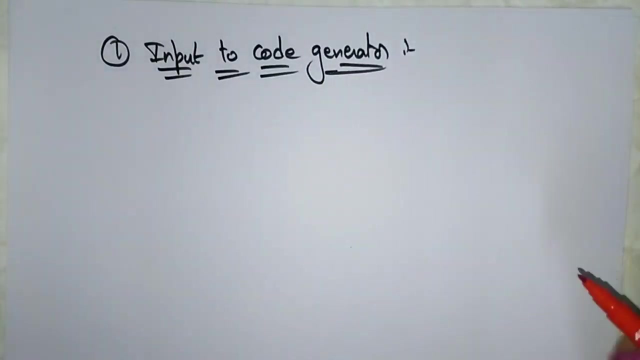 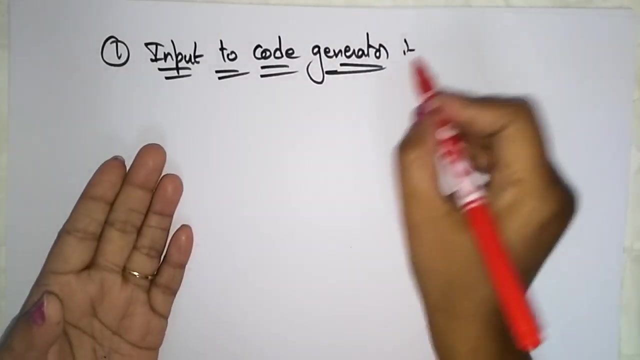 So this is one of the important question: try to know all the design issues of the code generator: input to code generator, So input to code generator. here the linear representation like post fix, and so I said the input to code generator is nothing, but you will get the intermediate code. okay, you will get. 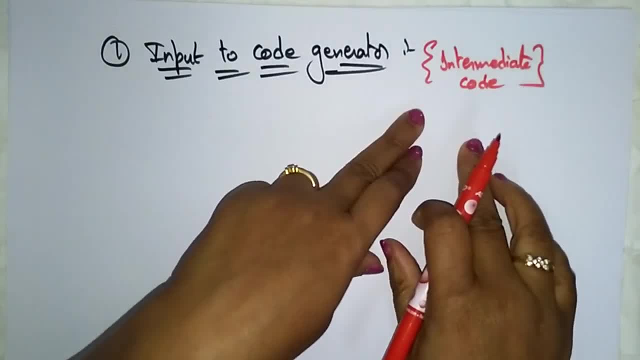 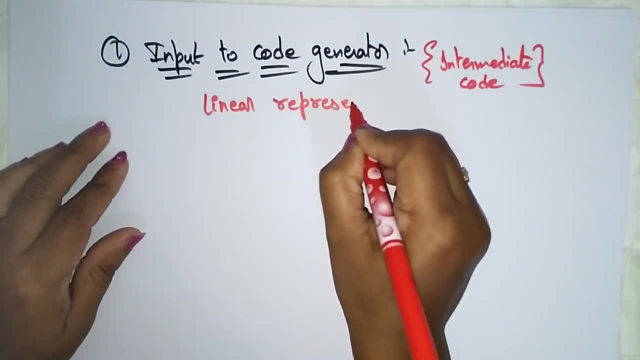 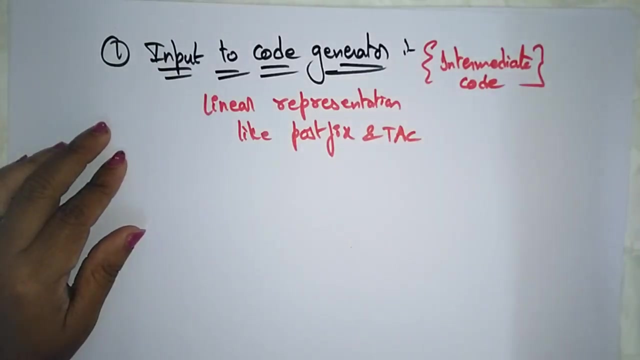 input as an intermediate code. so how this intermediate code will be, look, it's just a linear representation. linear representation like what you can say: The post fix expression, The post fix expression and three address code. the intermediate code is nothing but the output. here it is a three address code. 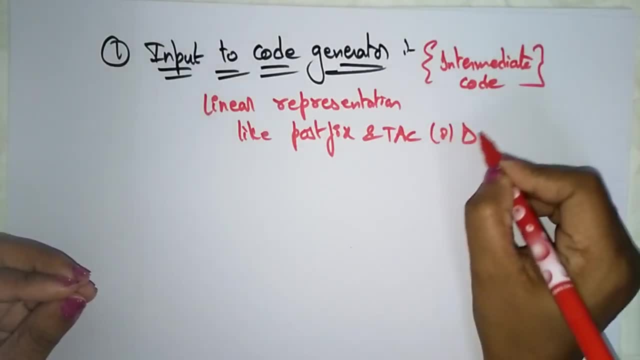 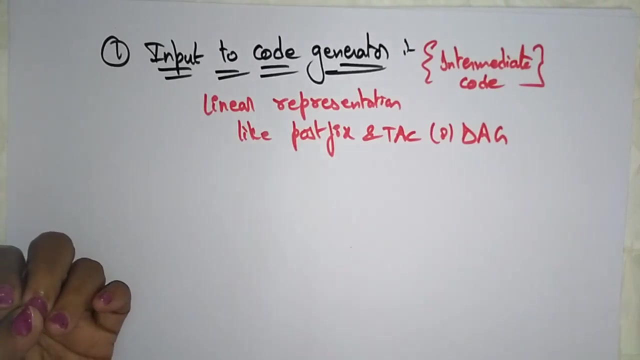 Or it may be represented as dag, directed as I click graph. okay, so this input may be any of these expressions. it is in the form of the intermediate code, is in the form of linear representation, like post fix three address code and the dag. Okay, and here you need to assume that type checking is done. okay, so in this representation that type checking is done and the input is free of errors. make sure that input is input is free of errors. 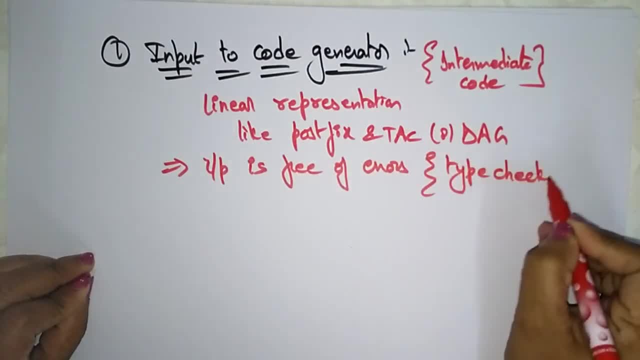 By performing the type checking. So the first design issue Is Is. The first thing is you have to give the input to code generator. so what type of input you are giving? it may be a linear representation. so while you are giving the linear representation, that is, an intermediate code, to the code generator, you have to be think the input is free of errors by performing the type checking. 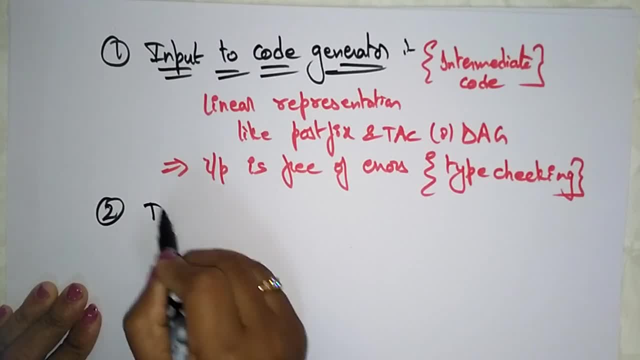 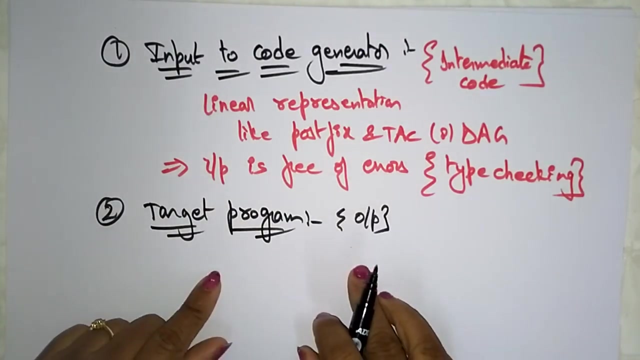 Now let's see the second design issue. so what is the second design issue? target program, Target Program. So the out here, the target program, is nothing but the out put Okay, the output may be many forms. the output may be many forms like absolute machine language. absolute machine language. the output may be relocatable machine language. 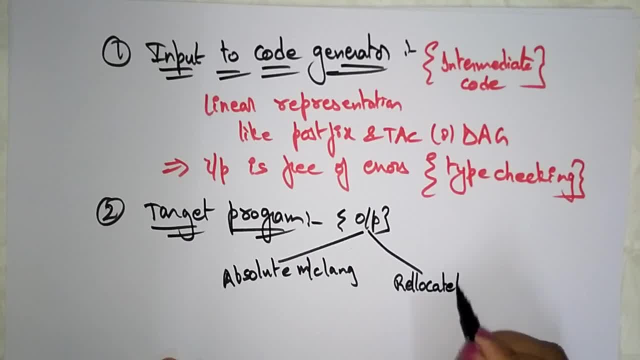 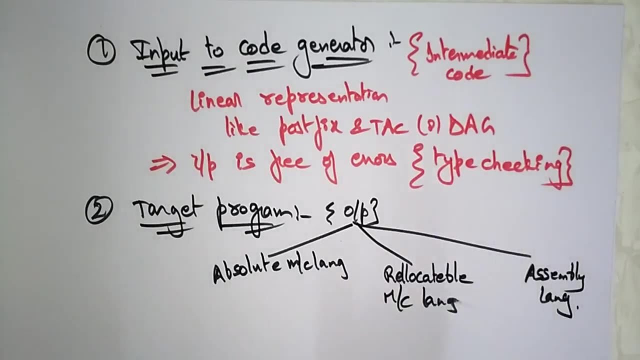 relocatable, relocatable machine language, or the output may be assembly language, so that is the target program. whatever you are generating, the output of the target program is the output for the code generator, so that target program may be in the form of absolute machine language, relocatable machine language and assembly language. 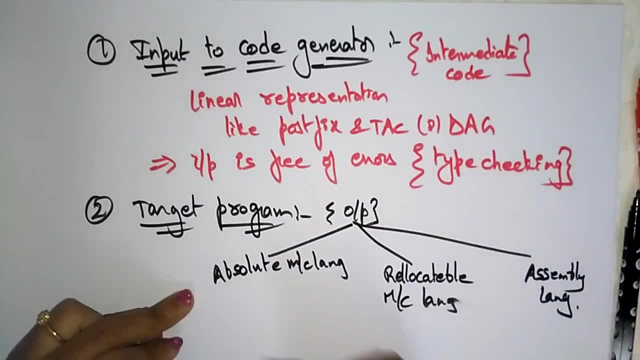 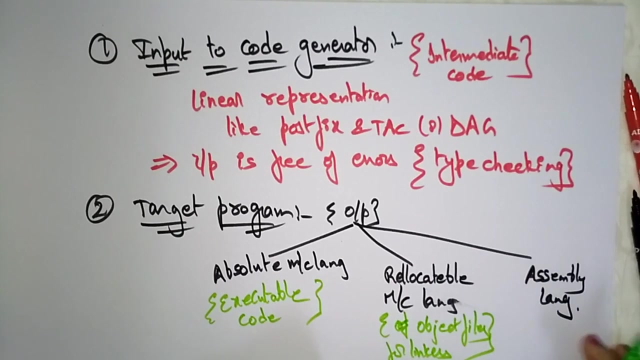 so the absolute machine language is nothing, but it is in the executable code, exe files. it is an executable code, so, whereas the relocatable machine language is like object files which are used for the linkers, object files for linkers. okay, and what about the assembly language? 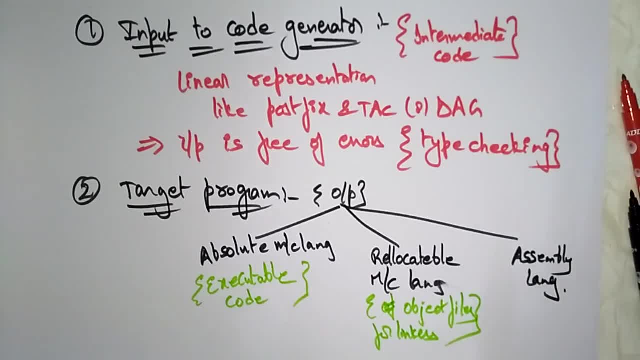 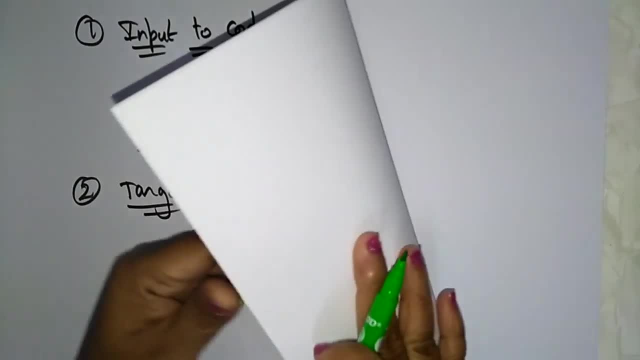 the assembly language facilitates the debuggers debugging. so this is a second design issue in the code generator. Now let's see what is the second design issue in the code generator. Now let's see what is the second design issue in the code generator. Let's see the third design, that is, a memory management. so memory management is one of. 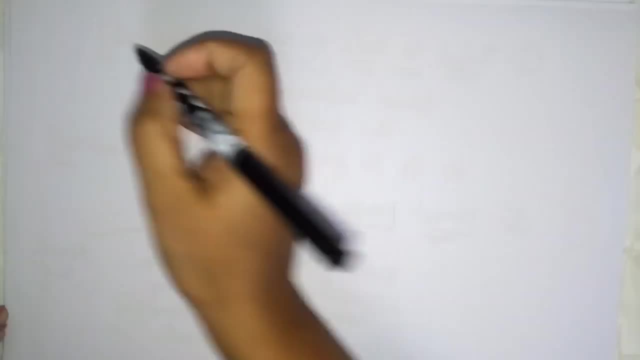 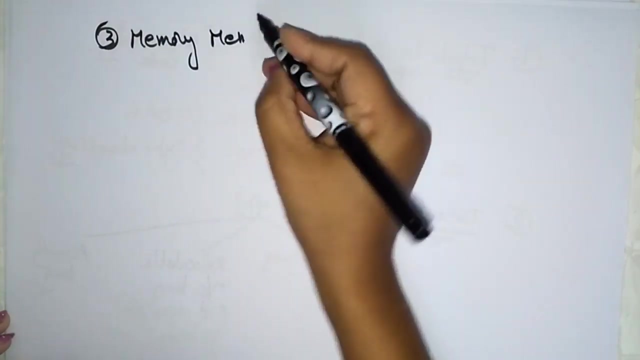 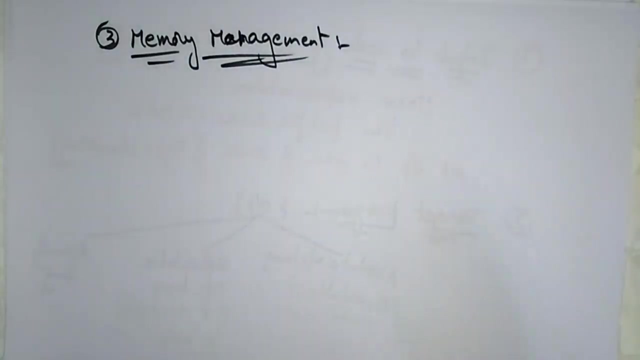 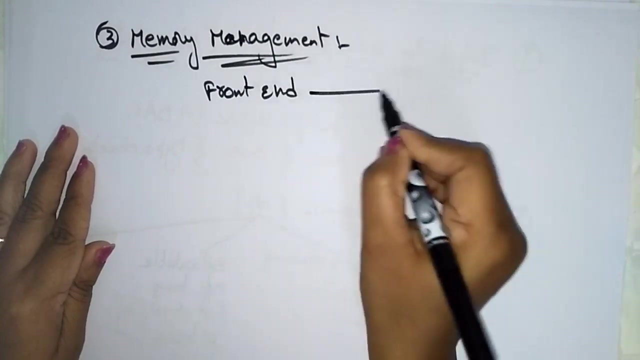 the big concept. in whatever the topic you are taking, the memory management is a management. so how the memory is managed in this code generator The mapping names in the source program to address of data object is done by front end. so front end is there, back end is there. we know that this is source program. 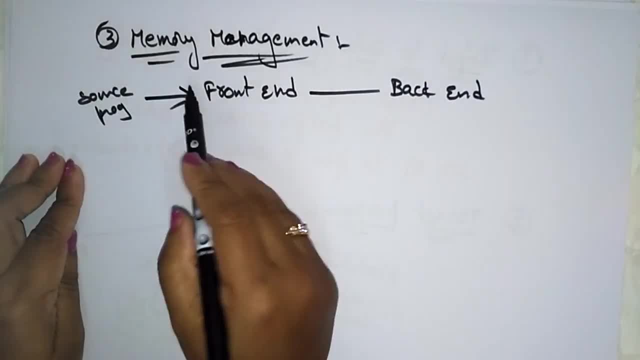 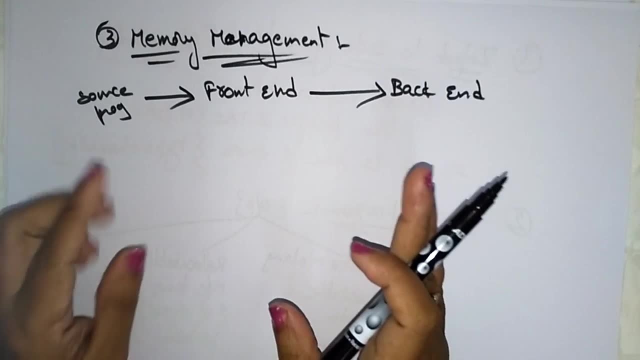 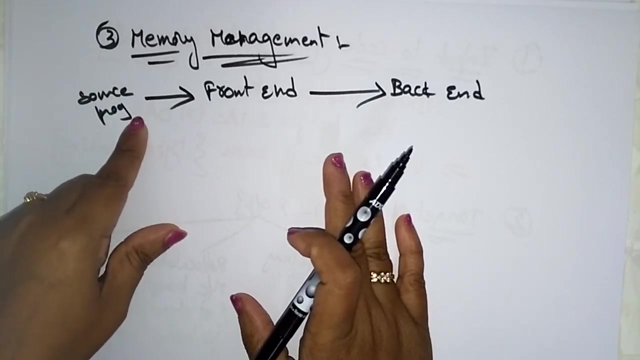 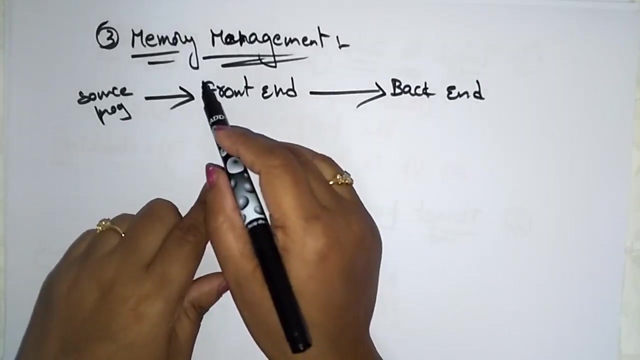 so the source program is entering into the front end. later it entered into the back end. okay, so in the compilation process that we know that. so here the mapping names in the source program. whatever the source program is there here the mapping names In source program to address of data object is done by in the front end. okay, so everything will be done in the front end. 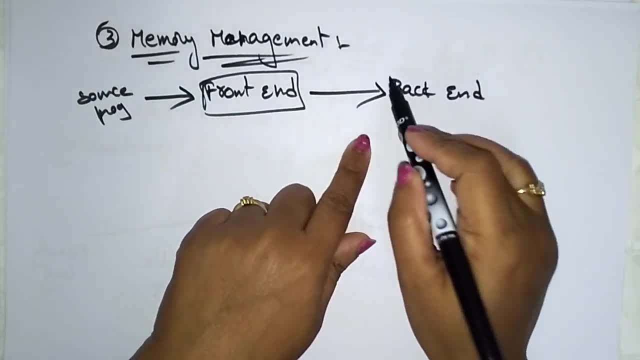 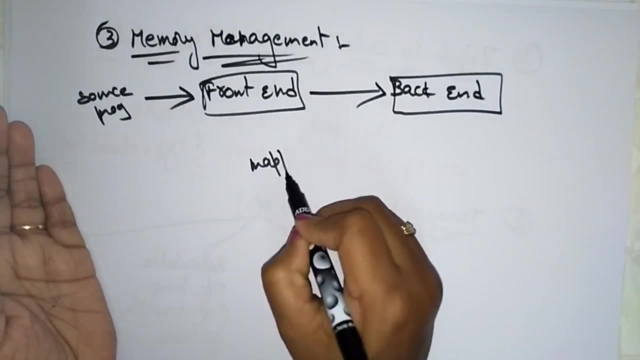 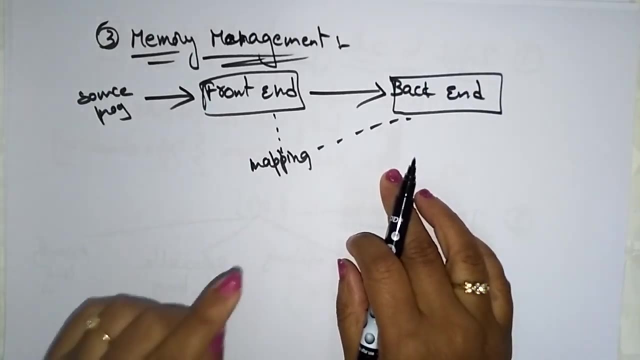 Front end and as well as the code generator also. so front end in the same way. in the back end also, okay, so the mapping can be done in both the front end, okay, and the back end. The name in three address statements. this refers to the symbol table entry for name: oh, 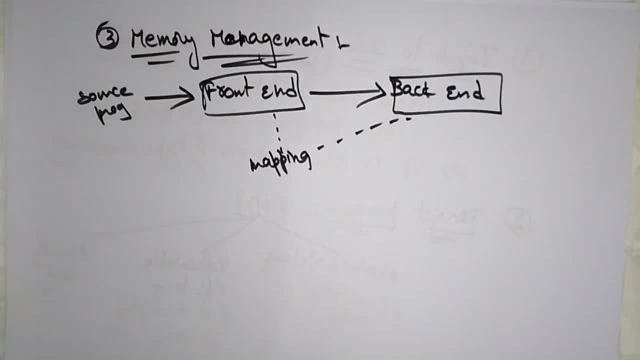 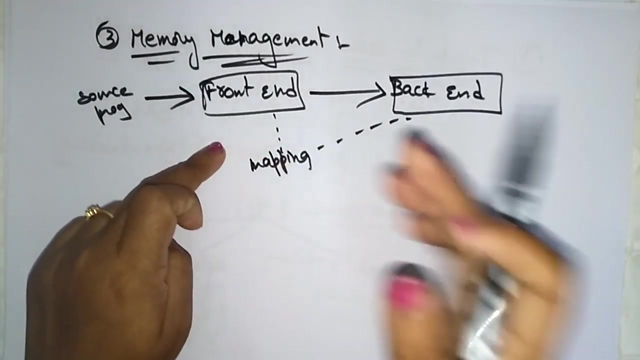 Lets take them from the symbol table entry. a relative address can be determined for the name. So here we are giving whatever the source program that will be there, so that will be sent. perform address of the data object is done by the front end as well as a back end. also, when every one you are using this type of objects, that address will be generated by front hand as well as a contain. whenever you are using this type of objects, that address will be generated by friend and as well as a back end. 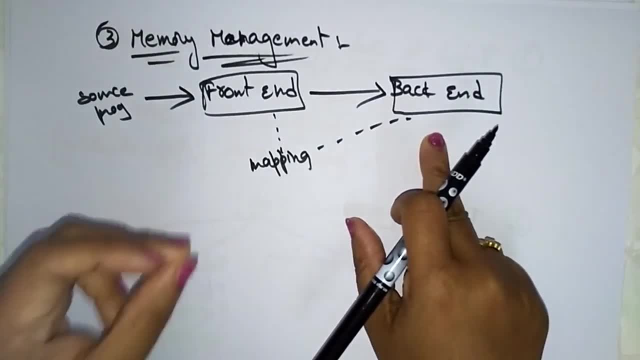 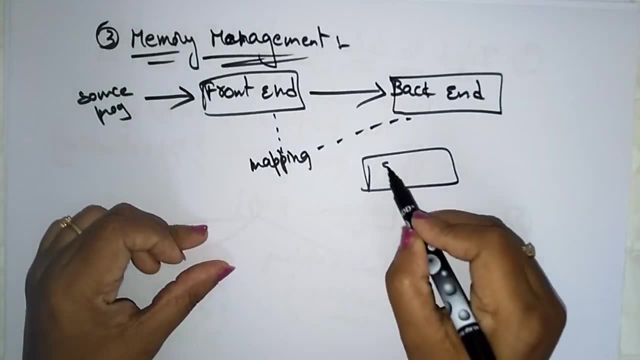 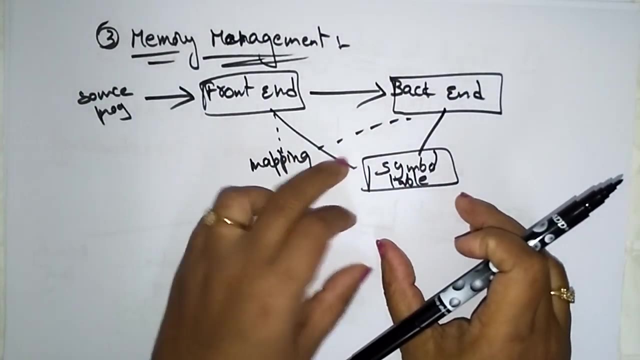 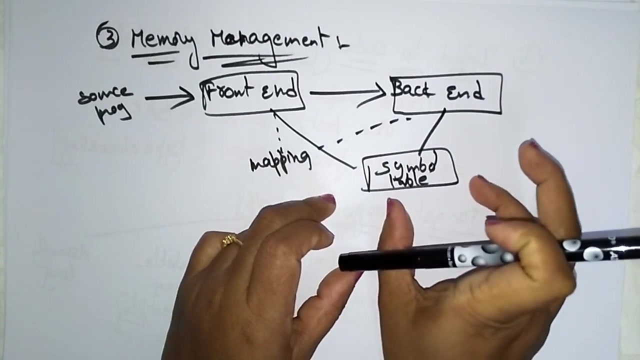 So this we can make. it is a good look. so Okay, now, any ways. back end also. so here, everything the information will be stored in the symbol table. okay, so the front end and the back end information regarding the variables information will be stored in the symbol table. so the symbol table: here entry, a relative address can be determined.